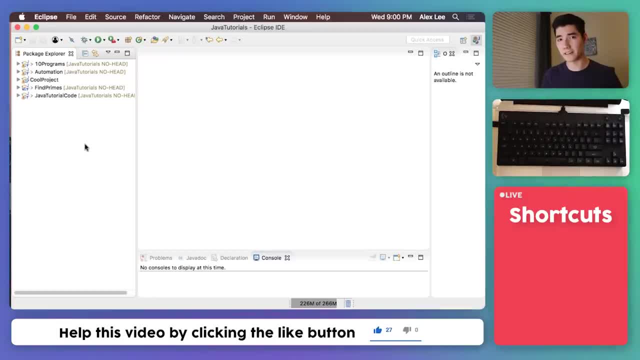 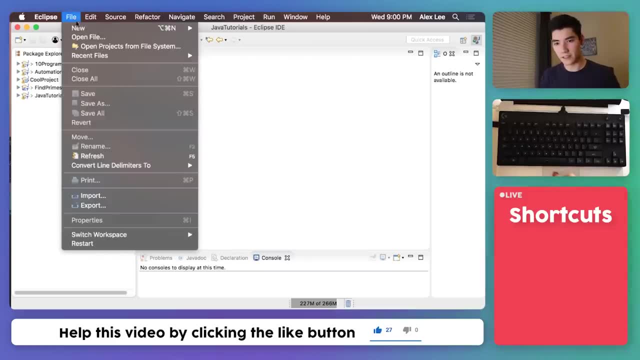 little bit. So if you're new here, you can go to the program. Eclipse or IntelliJ is a good one. I made a video of installing Eclipse on Mac and Windows. It's on the screen now. if you want to check that out. We'll just set up a file to start learning Java. So I'm just going to go to File. 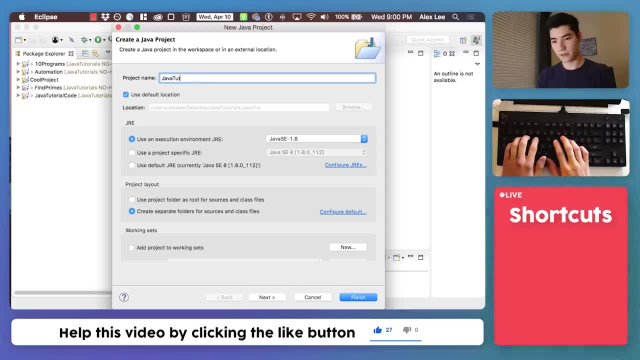 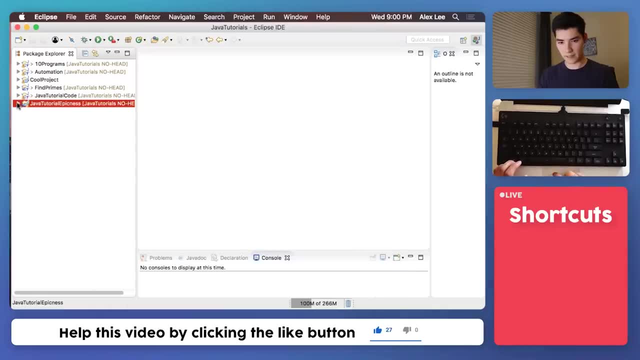 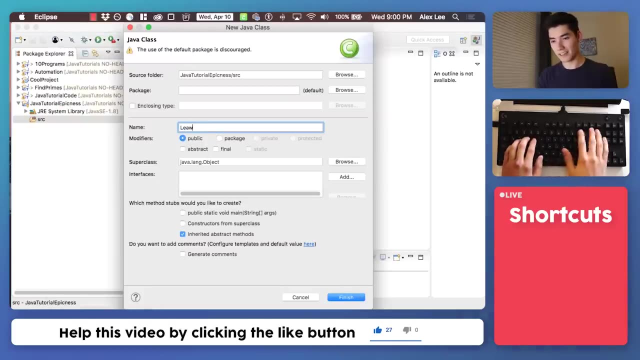 New Java Project. Type in the project name like Java Tutorial, Epicness. Hit Finish. Next expand that up, Right click on the source folder and go to New Class and this is just our Java name or Java file like Learn Java. Hit this first check mark Public Static Void Main and then hit. 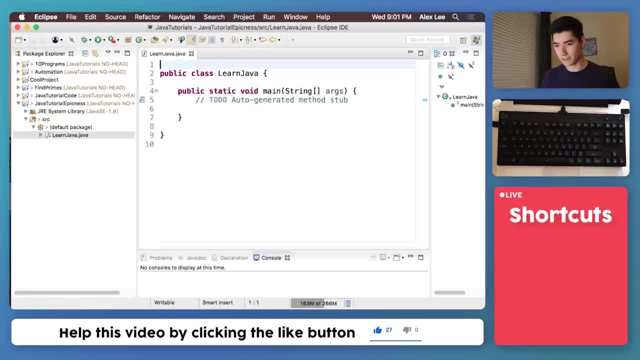 Finish And we get some code-looking stuff pop up on the screen. So, like I said, a programming language is just a bunch of keywords and symbols, and it looks like this Java file already has some keywords and symbols in here for us. A super useful thing we can do in Java is store data. 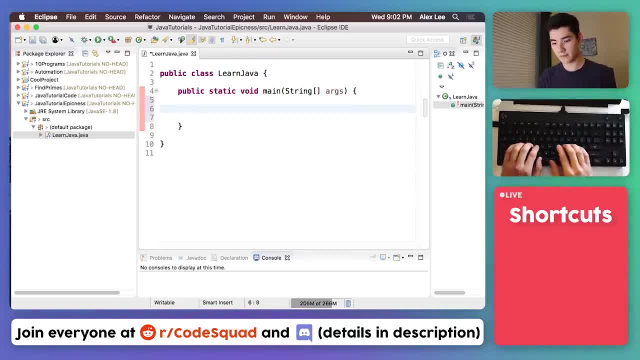 So you can store, say, a number variable in Java by doing this: Ints A equals say, 5.. This takes the value of 5 and stores it into A. You'll notice this keyword int- that stands for integer. And there are a bunch of other ones like I'm just going to list. 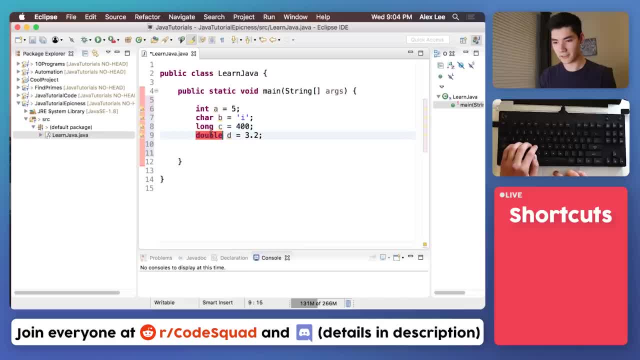 a few, So here's a few more. There's one called char long, and double Char stands for character. so this is how you would store a character variable: You would just put your character inside of single quotes and that would be stored into B. And we've got a few others like long. 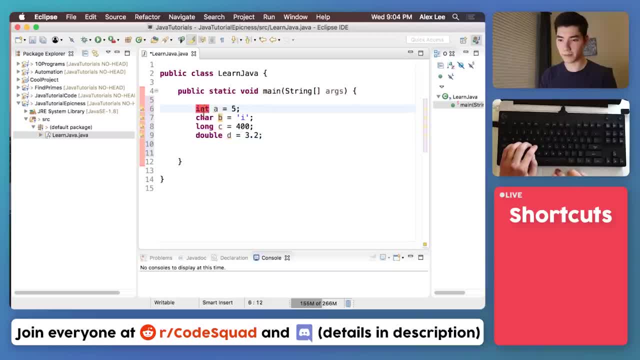 double and there are a bunch more. These are called primitive types since they turn purple, How primates are before humans. the word primary means number one. Primitive just means it was here before It's built into Java, which is pretty sweet. Let's go on to non-primitive types of. 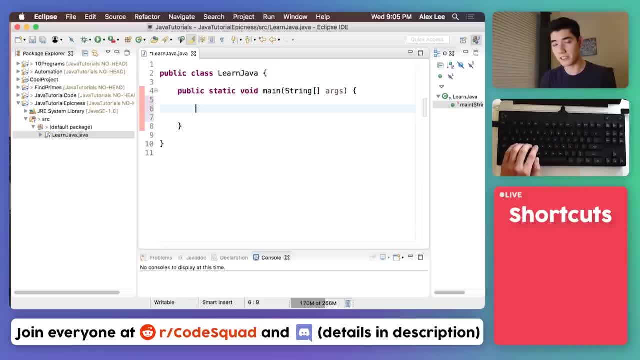 storing data, because storing data is super cool. If we wanted to change our username, say on Instagram, it's got to store it somehow, right? So to store a name like a bunch of character variables, that would be called string, with a capital S. there You'll name it like string name. 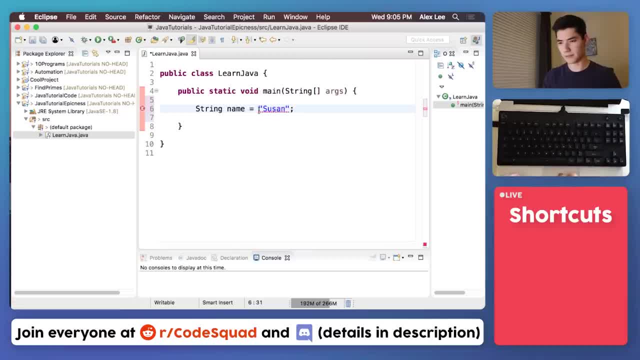 and set that equal to Susan and then put a semicolon at the end. Most statements will end in a semicolon. by the way, These don't for their own reasons, but if it doesn't have some sort of parenthesis at the end, put a semicolon there. All these symbols help Java parse it, which just. 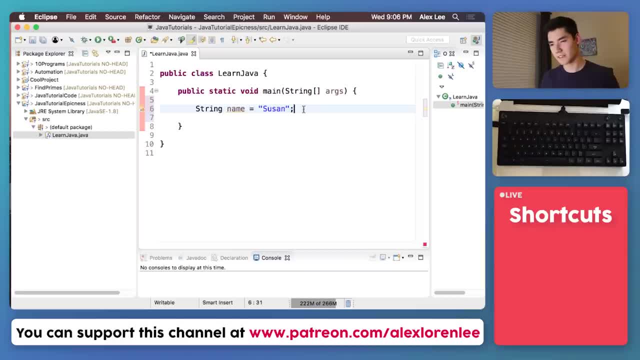 means go through and make sense of it all. So that's why these weird little semicolons exist. So now the name Susan is stored into name, but notice how this isn't turning purple. It's not a primitive type. If it's not turning purple, that probably means 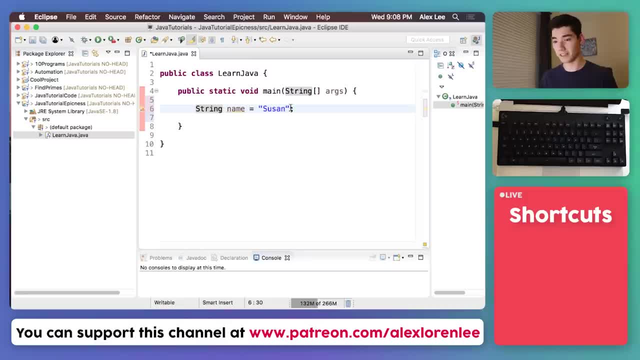 it's an object And you can do so many things with objects. it's crazy To do crazy things with your object. we can just type the name of the string, and in this case it's name. So we'll just type name. You'll see red underlines pop up. Don't worry about it. 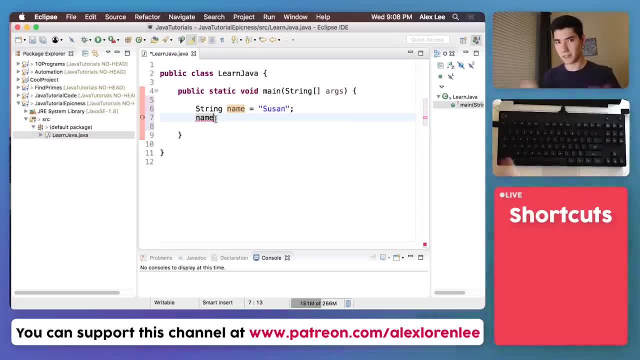 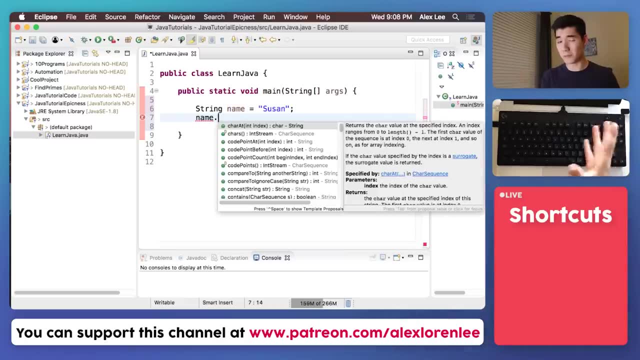 it's just trying to correct you before you make a mistake. I think it's really stupid because we're not done yet, But after you have the name of your variable, hit a period, And this period is maybe one of the most important symbols in Java because it tells you everything that that variable. 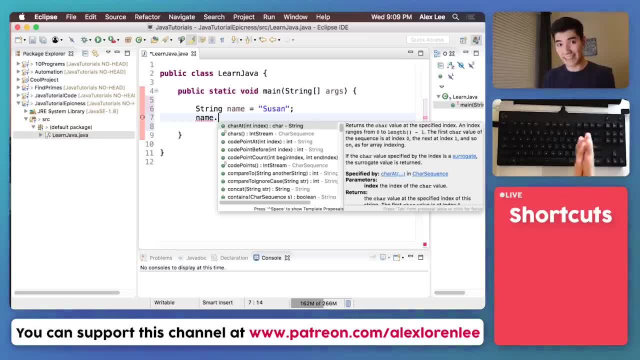 can do for you And it's a very, very important thing to keep in mind when you're writing JavaScript. you All that wonderful code built into Java. you have it accessed through this period. The programmer you're writing Java in will most likely have like a. 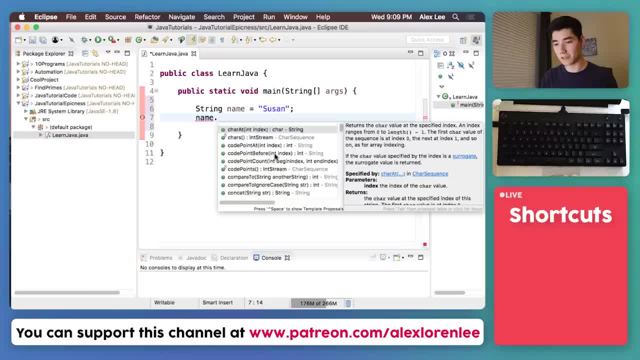 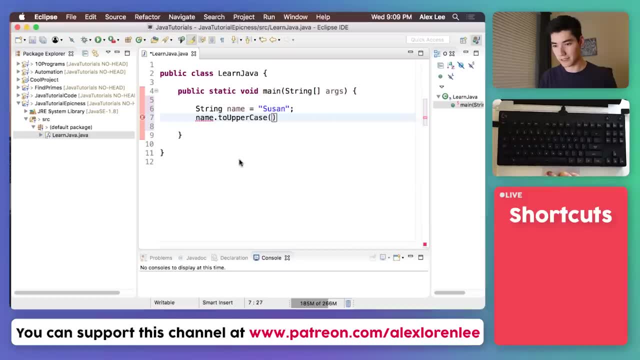 little box here and you can scroll through it, and this is everything you can do to that variable. So one I like to pick right now would be like to uppercase, So I can just double click on it, or you could type it out and then semicolon, since it's not opening a bracket. Well, how do we see this working? 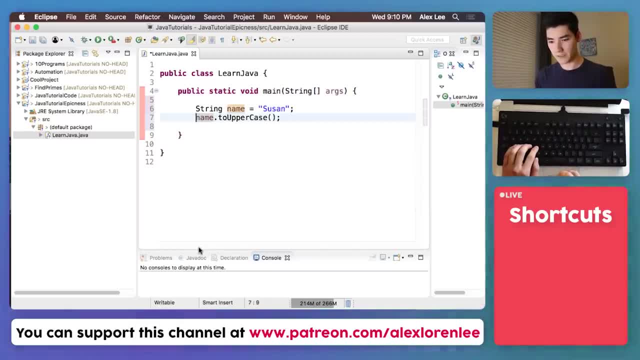 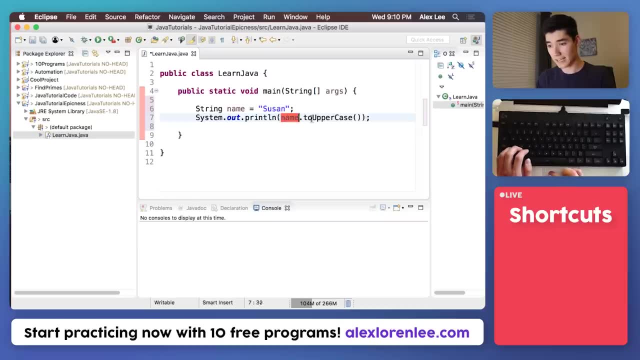 There's this great piece of code to print out so you can see things. It's called systemoutprintln and then some parentheses. We're pretty much just taking this and sticking it inside of the parentheses of this code. This just puts it on the screen for us. So I'm just gonna ctrl s or command s to save. 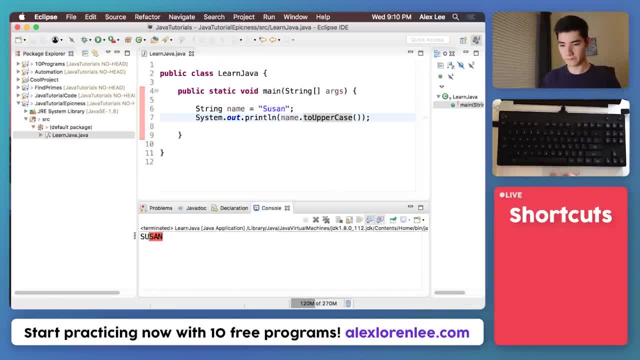 it and I'm gonna run it And then in your console window it might be called console, might be called something else, but in a window you should see a name to uppercase. If we want to see something else, we can just delete this. 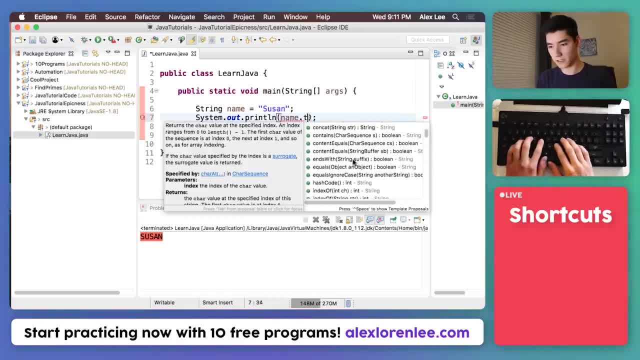 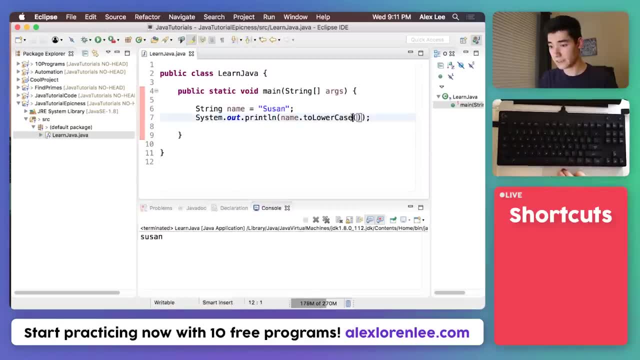 do the dot again to bring up what it can do. and there's one called to lowercase: Save it again, run it again and now it's all to lowercase. This to lowercase has some parentheses here and this putting text to the console window code has some. 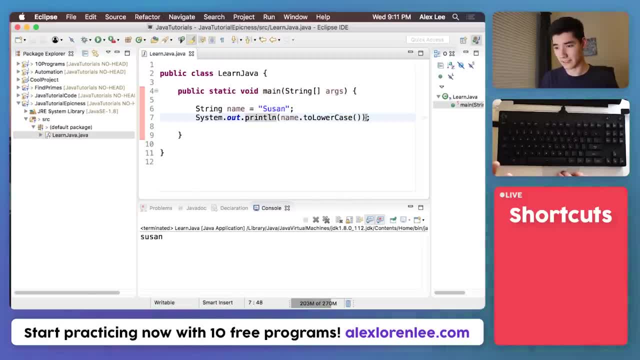 parentheses here too, And anything that has parentheses like this is, 99% of the time, gonna be a method, And methods are amazing. They're the, they're the, they're, they're the bomb, cause they just do things for you like, like what we did now. 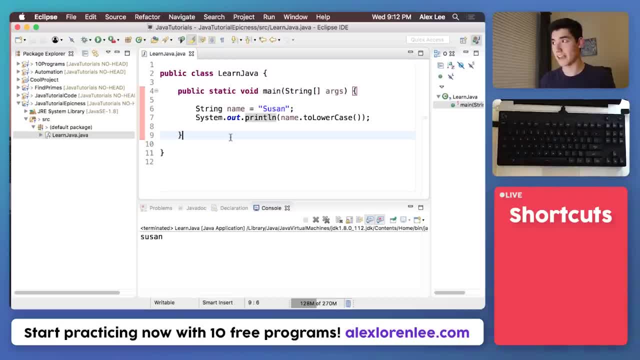 So let's make a method that puts an exclamation Mark, say, at the end of whatever string. you want To start a method, just write some keywords. We're gonna write the keywords: public, static void. Don't worry too much about this. right now They're just keywords and every keyword. 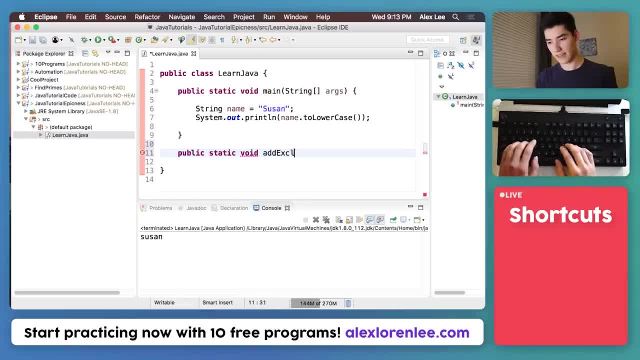 has its own purpose. We'll name it like: add x Clamation point. parentheses Say string s in here and there you go. knows what that is? Let's do it. We'll give it a new style: string s in here and then some curly braces to finish it off. I'm just going to delete these. 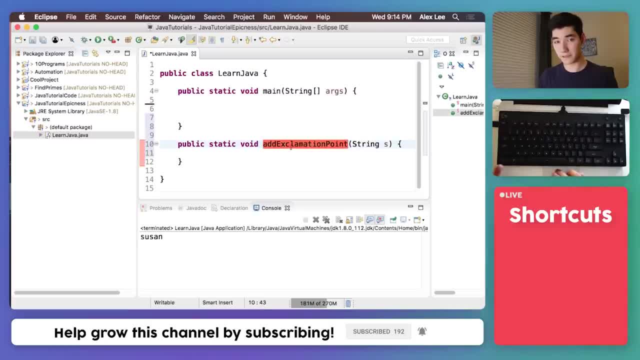 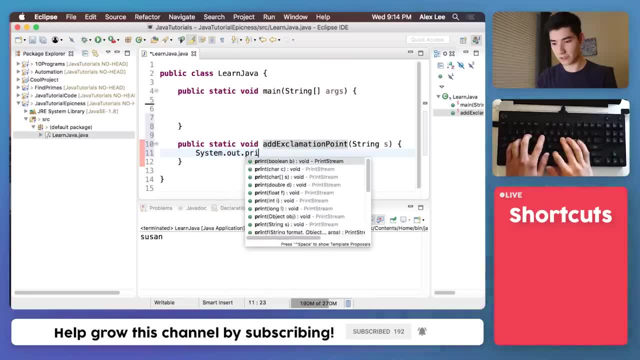 right now, because it might look a little confusing. All this method is going to do is add an exclamation point to the end, So we can just print out to the screen out like we did before. That's super useful To put two strings together. use a plus sign, So in the parentheses. 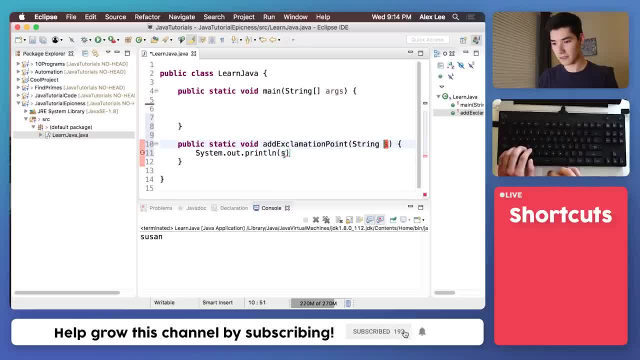 we'll just type s, which is the name of the string, plus an exclamation mark inside of double quotes, Since characters and strings- anything that's not a number or a variable name, has to be in quotation marks. Statements end in a semicolon. We'll save it and run it and nothing happens. 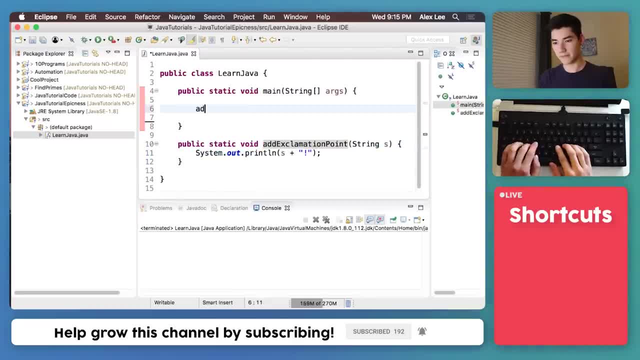 because we're not calling the method, So we'll just type the name of the method and then something like hot dogs. Now we can save it and run it, and we see hot dogs with an exclamation mark. This right here goes here and whatever's inside of these curly braces gets run. You can also 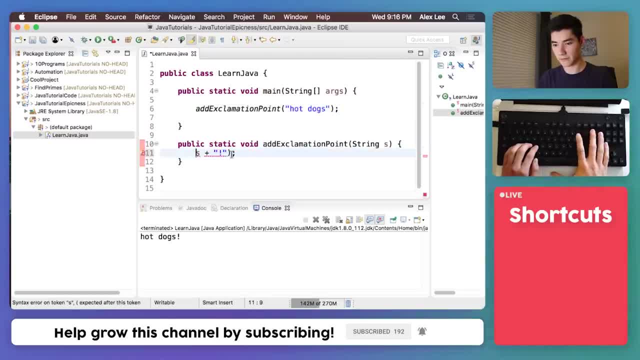 return the results as a variable. So we can say return, which is another keyword s plus the exclamation mark, You get a red underline because this keyword void is actually the type of what you want to bring back. So we just want to do a string and now we can say a string: exclaim is equal to. 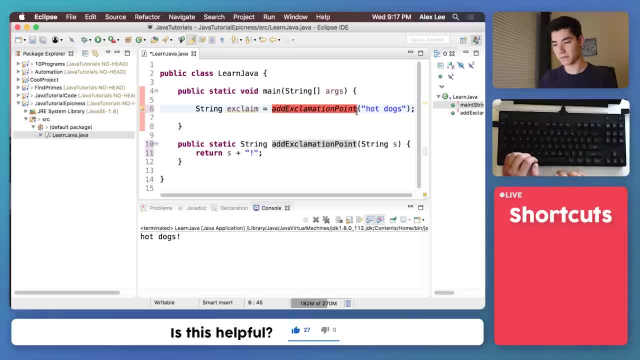 what's returned from add exclamation point. It's stored in here, but let's print it out and it does the same thing. As I said, the dot could bring up a bunch of methods that you could use. Well, you can also call them without a dot if it's in the same java file. But now I'm going to show you how to use code from: 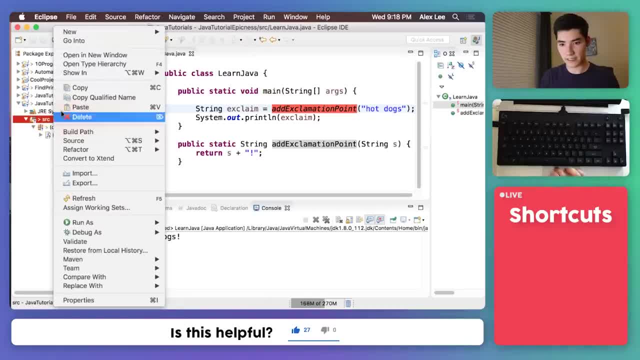 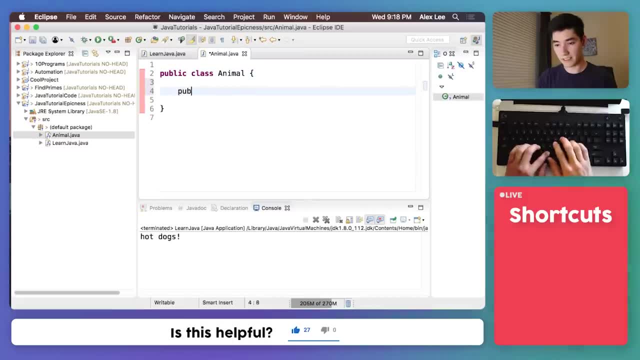 another java file into your java file. So I'll just right click source again, make a new class, We'll call it like animal and hit finish. I'll make a method just like we did before: Say like I am dog, and all it does is return I am a dog. If we want to use the 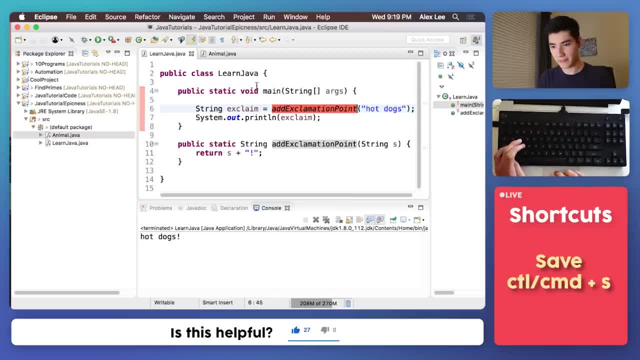 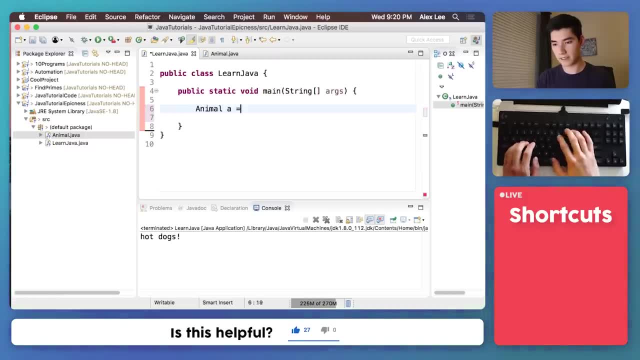 I am dog method. we can just- I'm just going to save it- go in here, delete this code for now To call I am dog. we can just make an animal object like this animal a equals new animal. Anytime you're making an object, it's going to have this format and there are a million types. 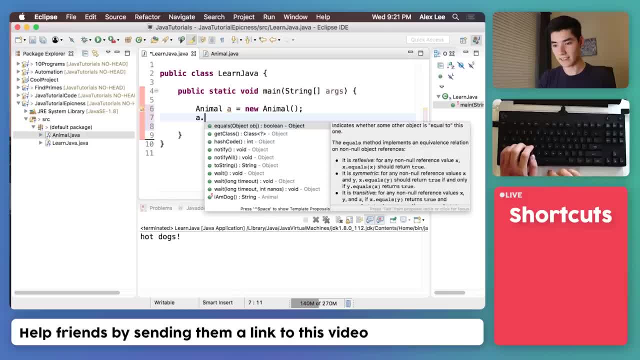 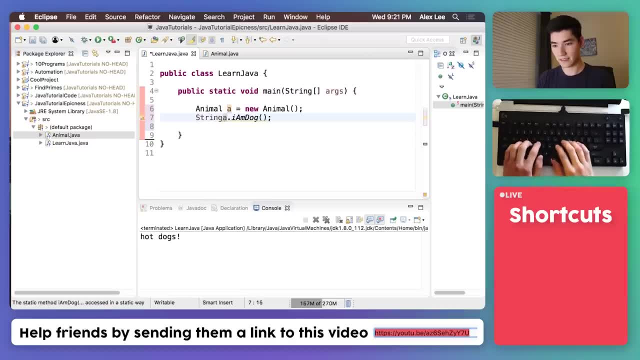 of objects out there you can use. But now we can just say a dot, and it brings up what that object can do and look, I am dog is here. We can just click it and then store that into a string So I am dog. and then print out dog, Save it and run it. and now you see that I am dog message. 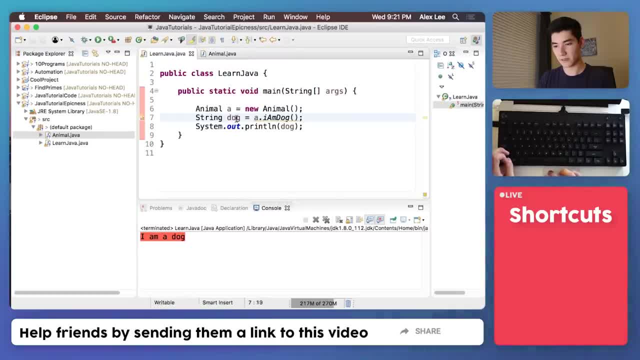 being returned to the variable dog. So a class is just a java file that helps us make objects. Examples of commonly used objects are: array list has the same format as before but you got to put these little angle brackets. But a lot of objects will not come in your code. You have to bring them. 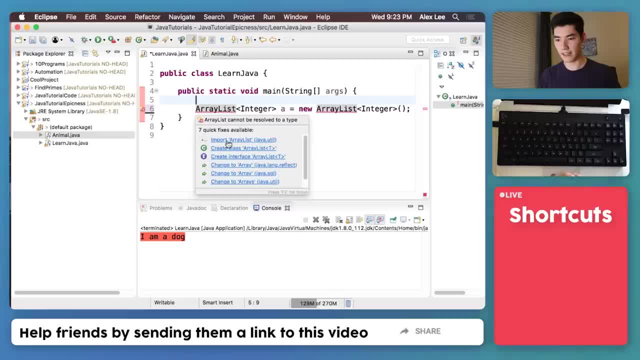 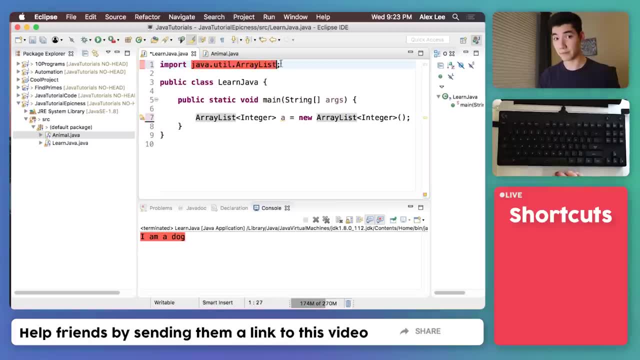 in. So usually what you'll do is hover over it and you'll see an import, Click the import suggestion and that'll generate this import keyword followed by like a path to the array list code. This just means bring the array list into our program so we can use it In array list you. 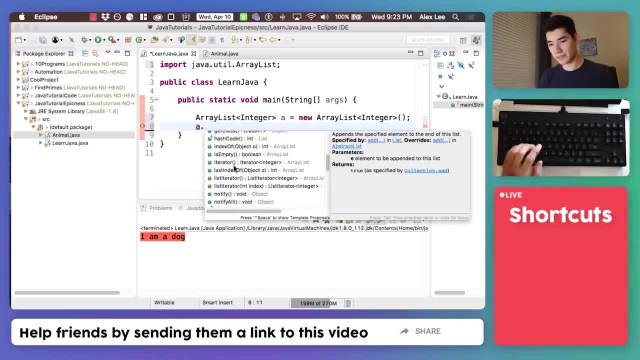 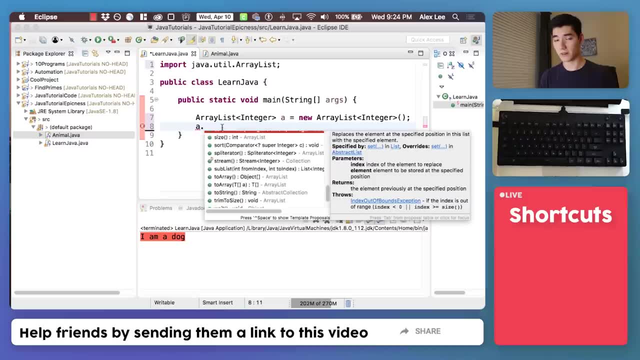 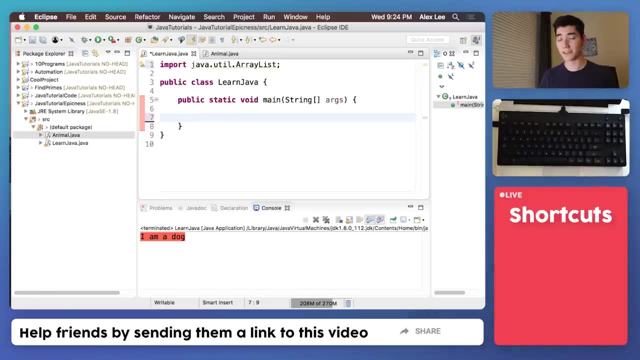 can do things like add. you can add a bunch of items like this is how they store movies, or store a list of users. You can replace that and all sorts of things. So objects and methods are super powerful. Each object has its own methods and that's why java is referred to as OOP, which is 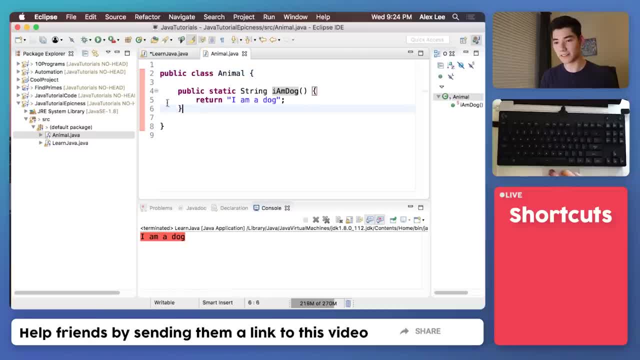 object oriented programming. Each class represents an object which has its own methods. like this one says: I am dog and you can add as many as you want. Now you might be asking: how do I make a method that does something actually cool? Well, we can start another one. We'll say void, since we don't. 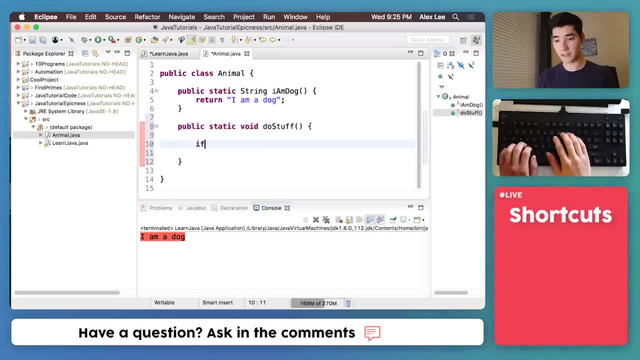 want to return anything. You can do logic in java. One keyword is: if This is called an if statement, You would have a condition in here Like true, and then it would run the code inside of here. This is useful if you have something like: 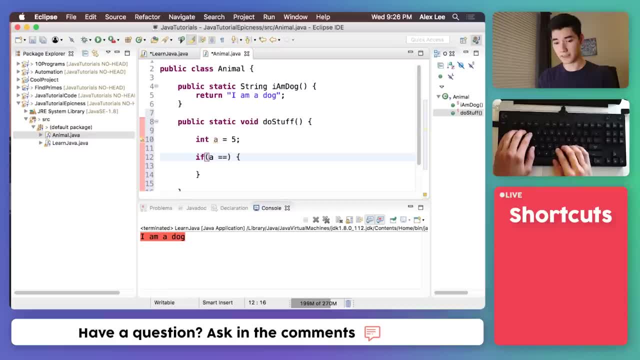 a is equal to a five, If a two equal signs. If a is equal to zero, then run this code. You can attack on another one Otherwise. if a is equal to one, then we want to run this code. Otherwise. if it's something else completely, then run this code. If all statements are super useful, You. 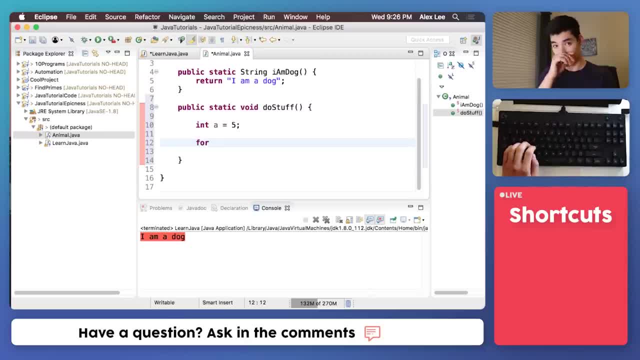 can repeat code by doing a for loop, and a for loop format has the keyword for it's in parentheses And then a format that kind of looks like this: In simple terms, this will repeat the code inside of here five times. You can change it, changing this number eight. It'll run this code eight times You. 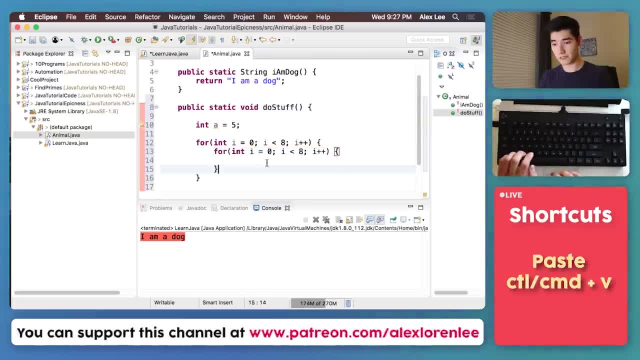 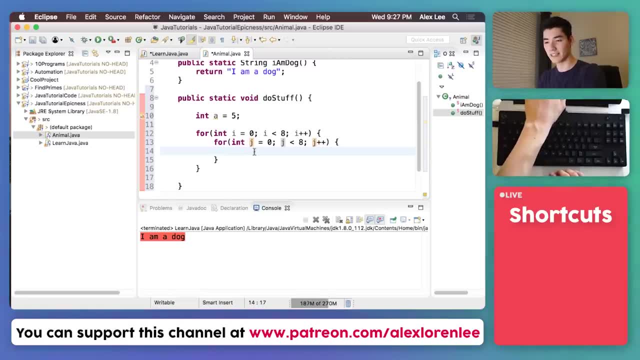 can put a for loop inside of a for loop, which makes it really interesting. Just gotta change this variable Now. whatever is in here will be run 64 times because it loops eight times and then another eight times inside. You can repeat code until a certain condition is met by typing: 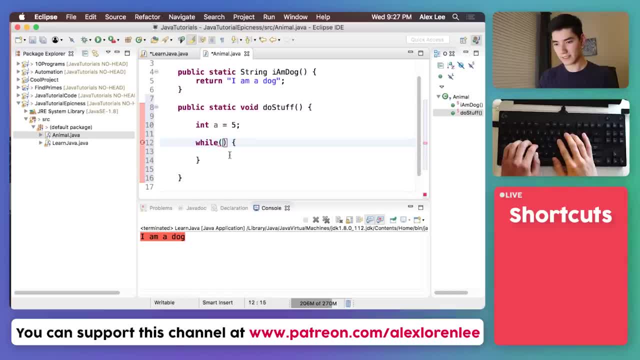 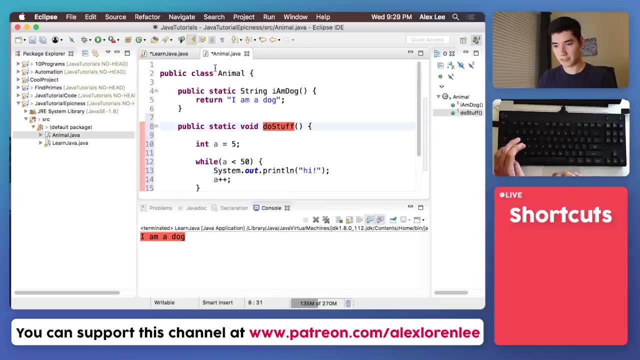 the keyword, while parentheses curly braces and say like: while a is equal to five, again print out high, it's actually. let's say: well, a is less than 50, print high and then increment a by one each time. that's what plus plus means. let's just call: do stuff so we can see what's going on. go into the main method. 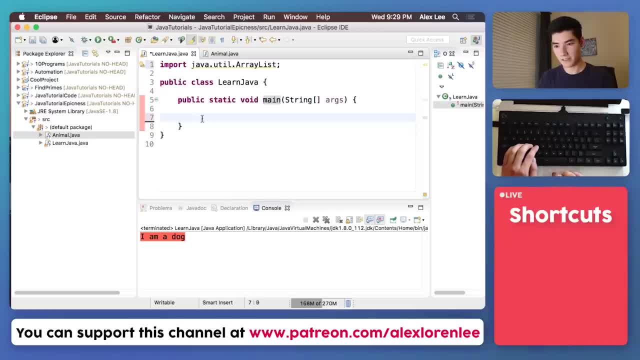 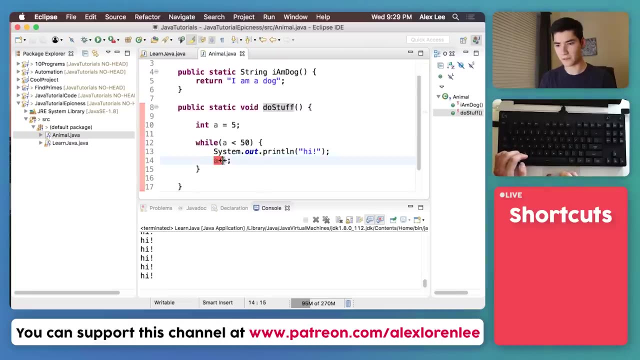 whatever's in the main method will get run when you click run. so we'll just make our animal again say a and then a period to bring out what we can do. and now we can see our do stuff method. if we run it we'll see high print out a lot and then it'll stop until it gets to 49 because it 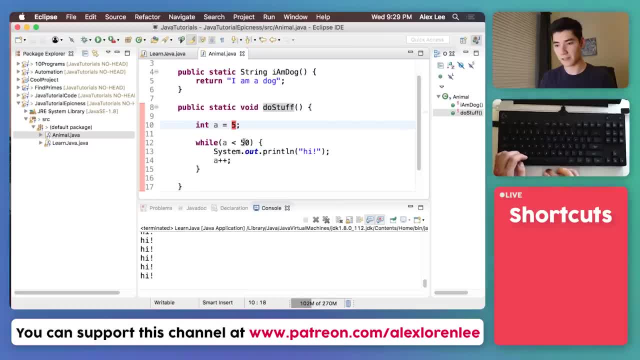 start at five, go up six, seven, eight, nine, all the way up until 50, and it'll stop. some other good logic ones are: try, catch, so the keyword try and then catch. it'll try to run the code inside of here. if something goes wrong, an exception is thrown. an exception means just something went.